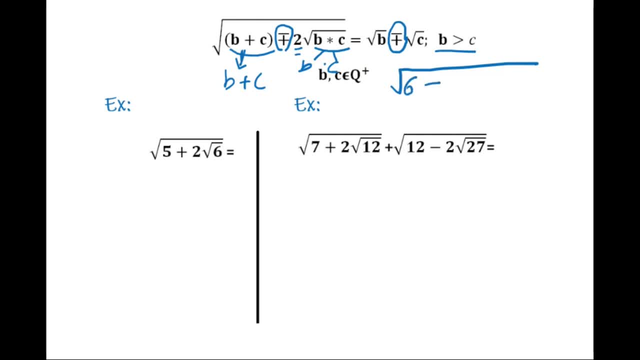 have six minus two square root of eight. if you look at this question, if we factor this eight as a multiplication of two numbers, let's say two times four, is eight, right, and if we add two by four, which is six, then we got the numbers that we are. 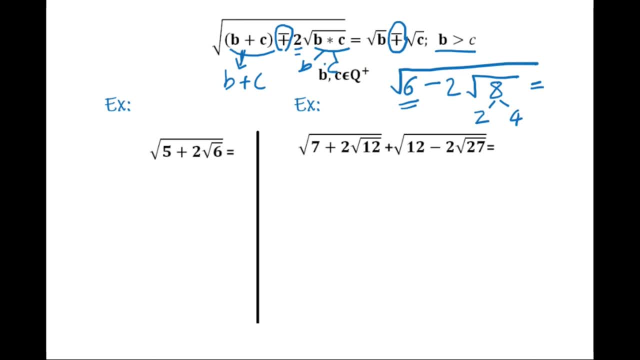 looking for. so this is equal to if you write the smallest one, first two, and then put it inside a square, and then the bigger one, second four, because there is a, the sign is negative. so just put the sign between them negative. so if you write this, okay, if 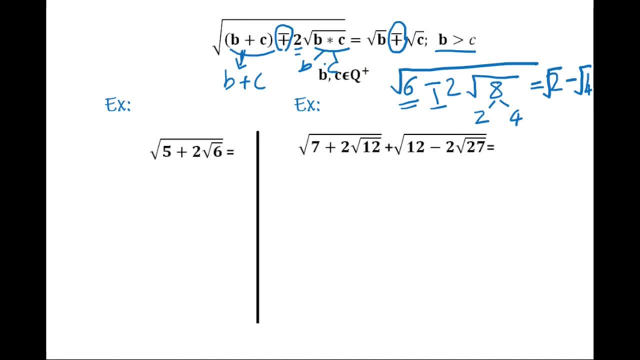 the result is square root of two minus square root of four. this is going to be a negative number. okay, because this is going to be a negative number. and this is a square root, the even root degree, because the left side has an even root degree, then there is not going to be there. the result cannot be a negative. 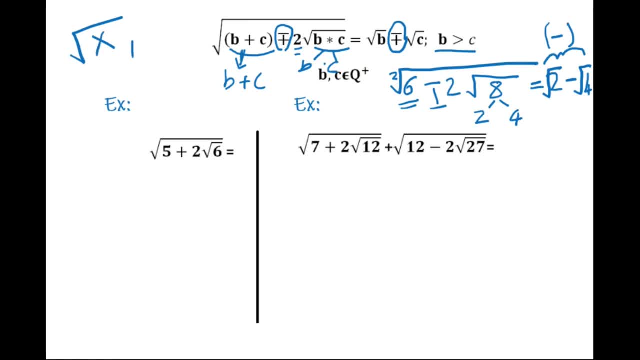 number. okay, let's say we have square root of X and we all know that that X has to be equal to greater than or equal to zero. so we should consider this and from this point of view of always- okay, this is not possible- always write the bigger one first. so square root of four minus square root of two and square root of four is: 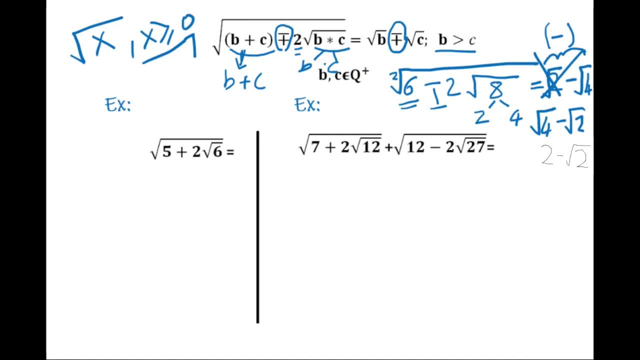 two. so the result is two minus square root of two anyway. so if there is such an expression, okay, there are some criteria, certain requirements. in order to write the right side in this form. what they are? well, there has to be two in front of two second roots. okay, it is a must. so let's. 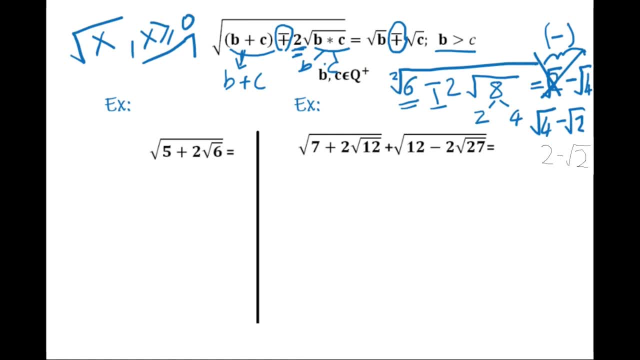 take a look at our first example. here, for example, we have square root of five plus two times square root of six. if you factor this in all, it is six, like two times 3. right, we can make it: two times three is about six, and if we add them up it's gonna be five. so this is equal to write the. 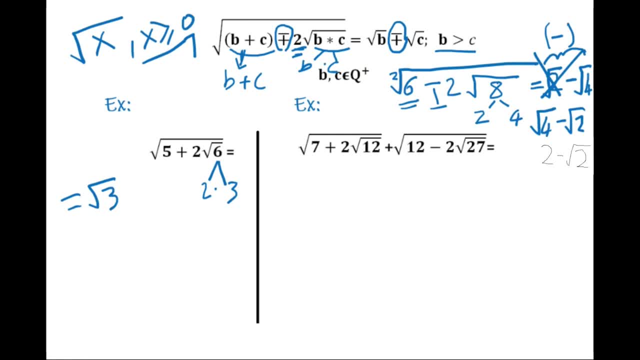 bigger one, which is 3, and put it inside the root, so score square root of three. and because the sign which is between the terms is positive or plus, so put here plus. and the second number, 2, so put it here plus. right, it is positive or plus. say if our 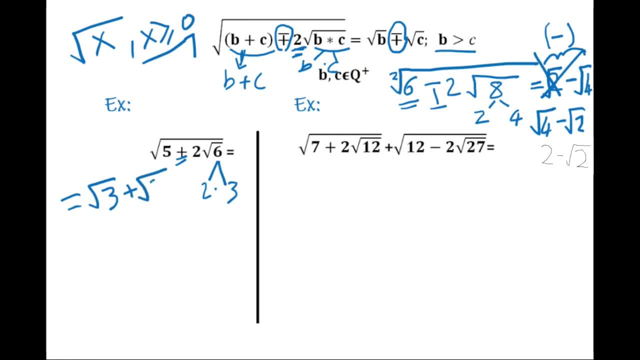 from this here, and the sign which is between the terms is positive or plus. so it is positive or positive, so put it here: plus, and the second it inside the rule. so the result is square root of three plus square root of two. you would say that you would factor this: okay, six, like six times one. this is also another case, but here if you add six, 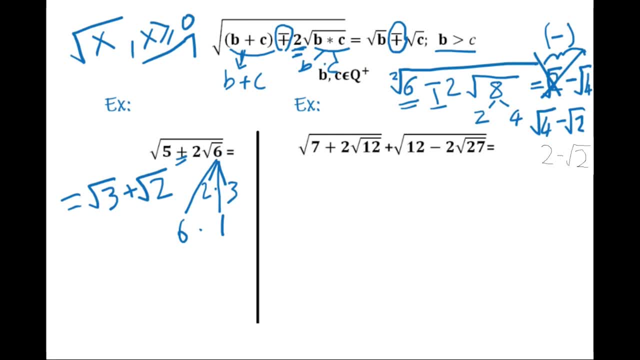 by one, it's not gonna be equal to five, so you cannot consider this case. if you factor that number, which is six we have here, okay, and the addition of these numbers has to be equal to the first number that we have here. so in this first question we have the answer. 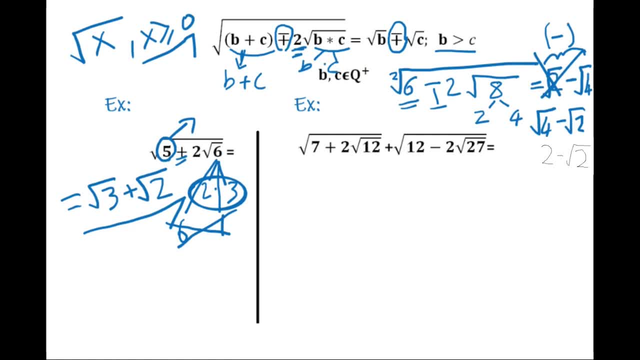 is square root of 3 plus square root of 2.and let's take a look at the second case that we have on the right side. we have square root of 7 plus 2 times square root of 12 plus square interact stored example investigation. 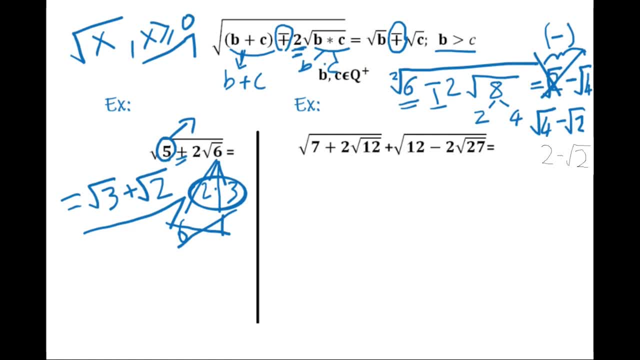 of 12 minus 2 times square root of 27, and what is the result of this? we see that we have two here. okay, and then we have two here, so our first condition is satisfied. that means we can factor the number that is very inside. okay, as we can write this number as a multiplication of two. 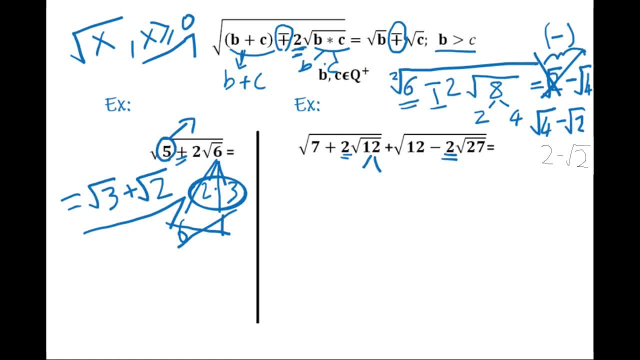 numbers and we have to consider that the sum of these two numbers has to be equal to seven. so if you factor 12, as for example 2 times 6, because 2 times 6 is 12, but if you add 2 by 6 it's not going. 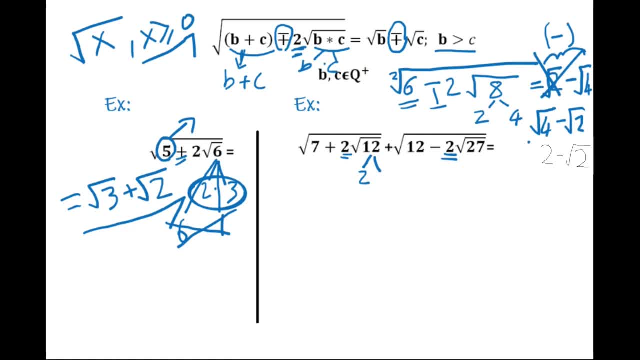 to be equal to 7. okay, so this is not going to work. how we can factor 12? well, we can write 12 as 4 times 3, right? because if you multiply 4 by 3, it's going to be 12, and if you add 4 by 3. 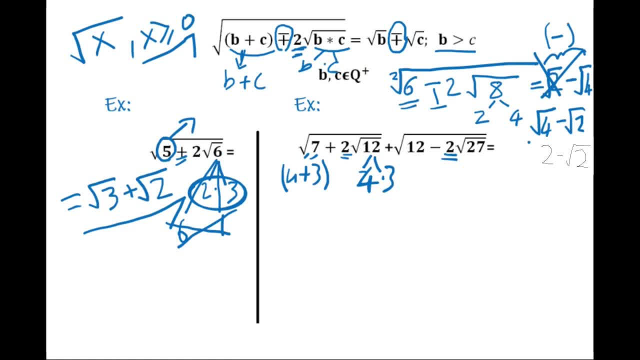 this is 7, right, it is equal to the first term that we have for the first square root. okay, for this one we have square root of 4 and because the sign is that is between is plus, so i'm going to put here: plus square root of 3 plus, and we have to factor this 27. 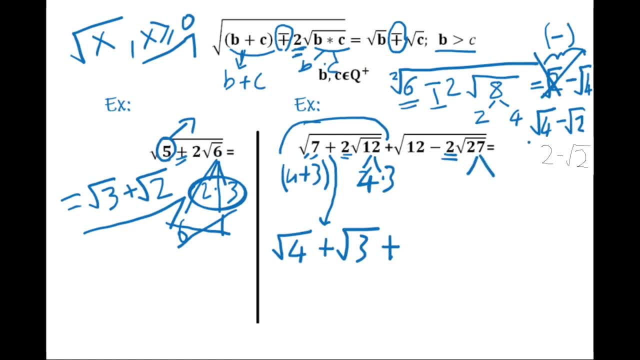 as a multiplication of two numbers. so if you multiply 9 by 3, it's going to be 27 and at the same time, if you add 9 to 3, okay, 9 plus 3 is 12. that means you can write the second term as square root of 9. i am always writing the bigger one first, okay. 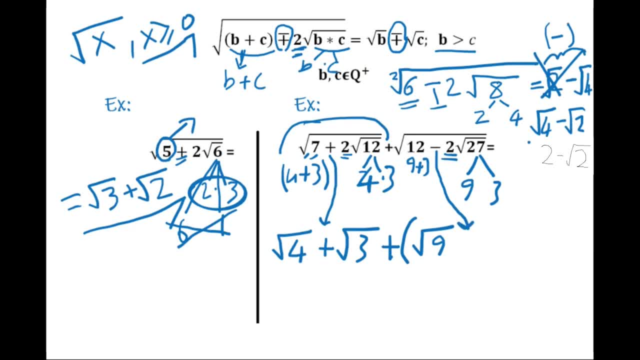 and the sign which is between the term, the roots, okay, the numbers. it is negative. so i'm going to put here: minus square root of 3.. and now the second term is minus square root of 3.. and now this is what we have. well, we can open these parentheses and then write down the expressions. 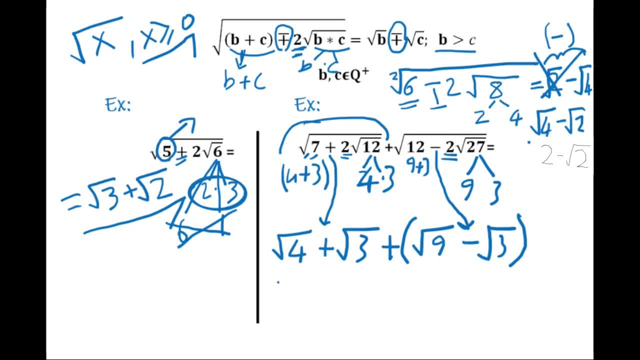 we all know that square root of 4 is what 2. we all have learned this from our previous videos. so 2 plus square root of 3 plus square root of 9 is about 3 minus square root of 3. why? because mine plus times negative is going to be negative. so here, if you add 2 to the 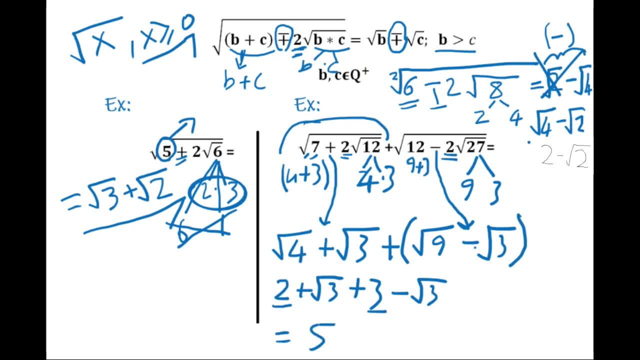 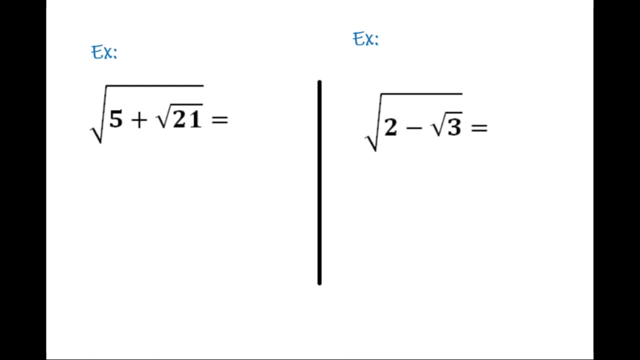 to three, we're gonna have five. this is positive square root of three. this is negative square root of three, so we can cross them out and the left over is square root of five. so the final answer is square root of five in this case. we have two more examples, but here in these questions we see that there is 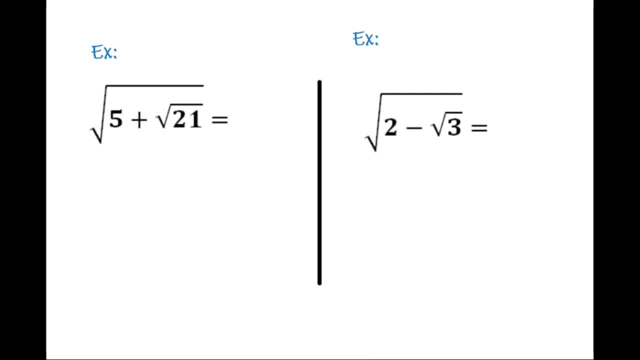 no two. what if there is no two? in front of the second rule and what we're gonna do in order to apply the method that we have learned in this video, there is a must, which is there has to be two right here, right. so i am putting here two divided by two. 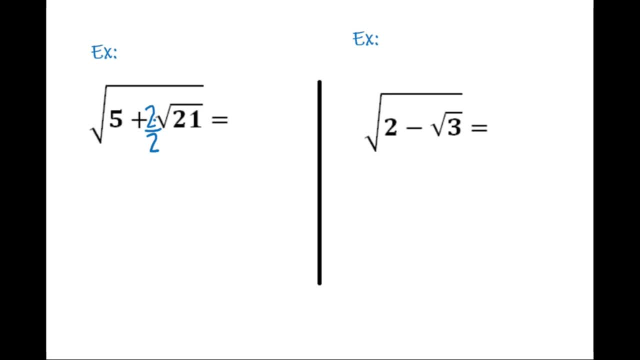 so in this case, in the next step, i'm gonna write the expression like this: five plus- i'm gonna keep the first two inside, okay. and then i'm gonna write the expression like this: five plus, i'm gonna keep the first two inside, okay. and then i'm gonna put one divided by two. 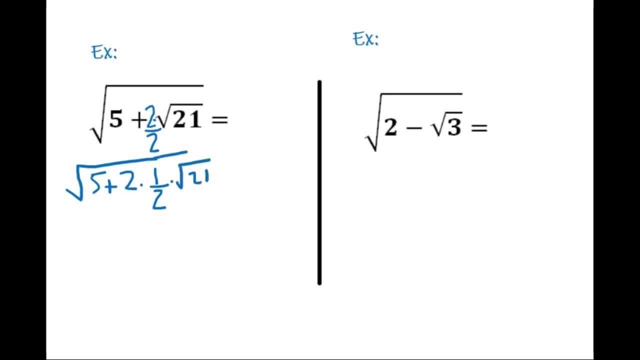 times square root of twenty one. so what i'm gonna do is i'm gonna keep this two, okay, in front of root and then i'm gonna send this one divided by two inside the root, okay, so this is gonna be equal to guys square root of five, plus now there is two times square root of. 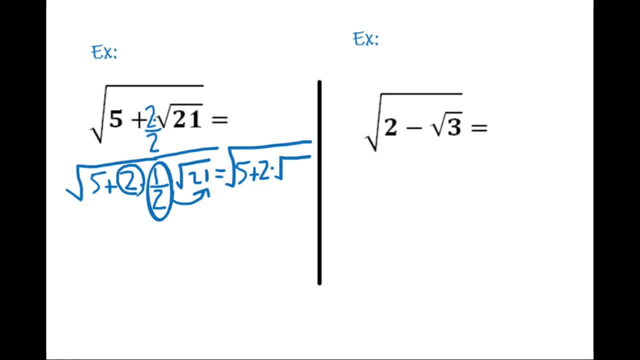 when this one divided by two comes inside, then it's gonna it becomes one divided by four. right, because if you think one divided by four, if you send it to the other side, it's gonna be one divided by two. so you need to follow the same thing in. 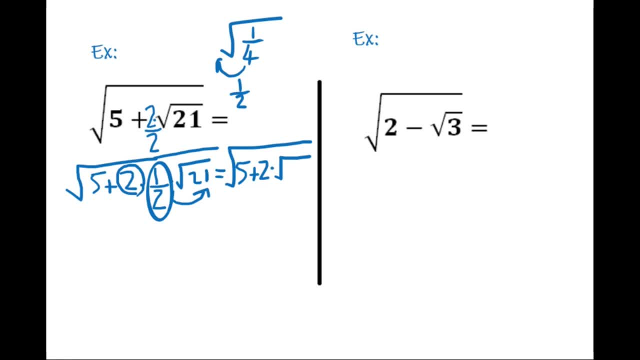 the reverse order. okay, once you send one divided by two to the inside of a root, then it becomes one divided by four. so it's gonna be one divided by four times twenty one. okay, then it's gonna be twenty one divided by four. the root is this. so, and now? in this case, we 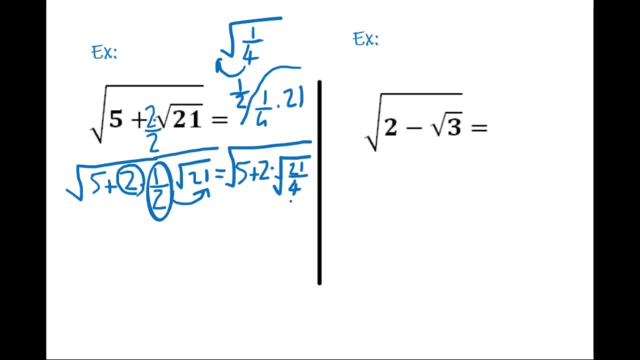 need to factor twenty one divided by four. okay, we need to write it as a multiplication of two numbers. so if we can write, okay, let's say we have three divided by two times seven divided by two. right, if you multiply it: three divided by two by seven. 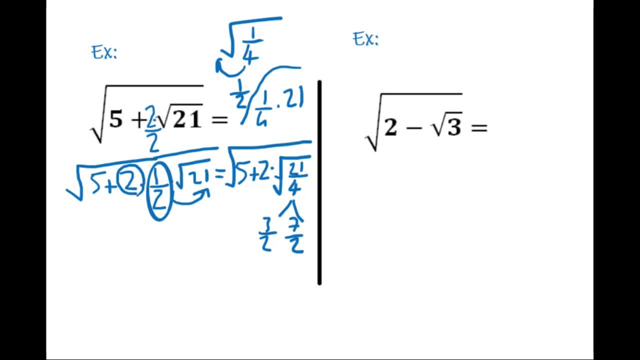 divided by two, then we have twenty one divided by four. so if we add three divided by two, by seven divided by two, and as you can see, the denominators are same, so we can add the numerators: three plus seven is ten, so it's going to be ten divided by two. 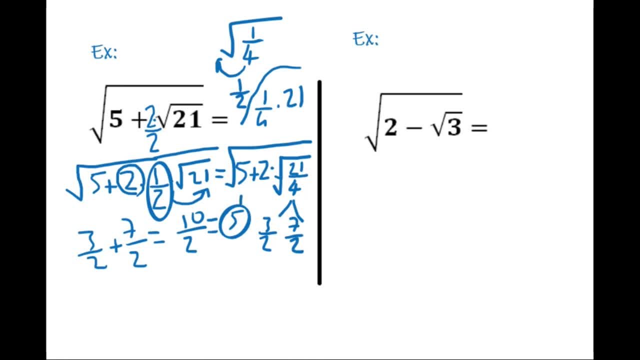 which is five, which gives us the number that we have as a first term. okay. inside the root, that means we can get the number of the last three, okay, okay. so the whole expression is okay, let me write it here: square root of five plus two. square root of twenty one divided by: 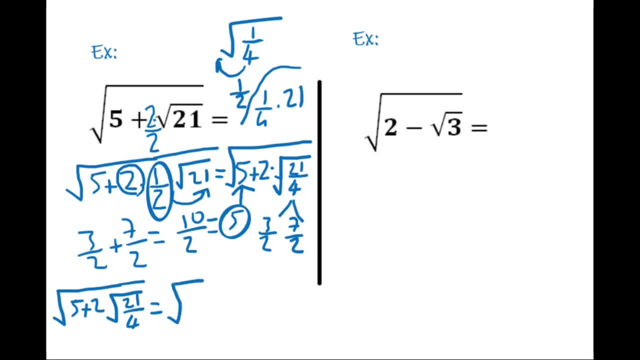 four is okay, square root of always. i'm writing the bigger one first. okay, seven divided by two plus square root of three divided by two, And you can write this expression also as square root of 7 divided by square root of 2, plus square root of 3 divided by square root of 2.. 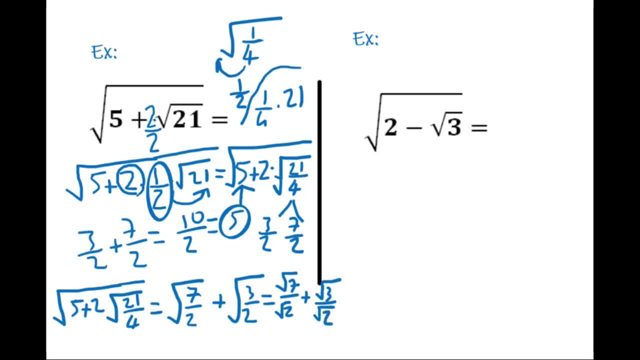 In roots. if there is a root in the denominator, then we need to get rid of that too. This is the general method that is applied in the roots and radicals. So how we can get rid of this square root of 2, well, just multiply it by itself. 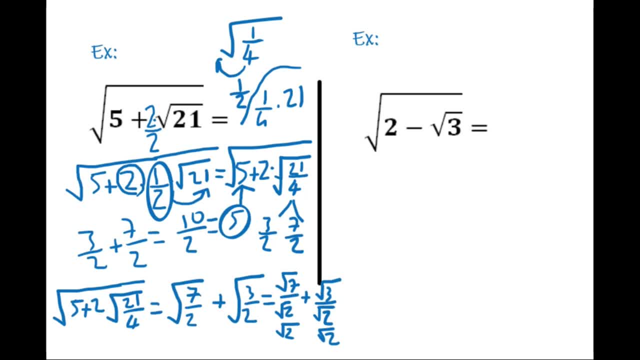 So square root of 2 times square root of 7, let me write it here- square root of 14 divided by square root of 2 times square root of 2, which is square root of 4, which comes out as 2, plus square root of 2 times square root of 3, which is square root of 6, divided by: 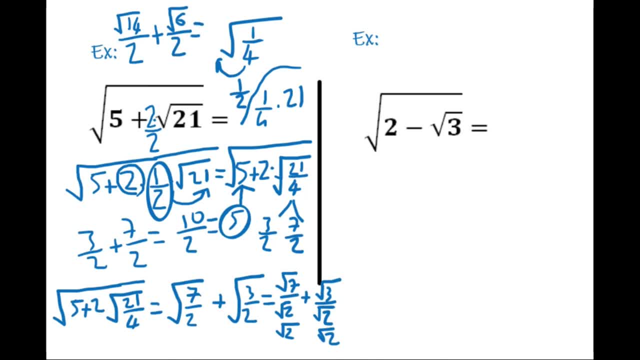 again, We have another 2, because the denominators are the same. so we just add the numerators, which gives us the answer as square root of 14 plus square root of 6 divided by 2.. This is the final answer, guys. This is the result of the question. 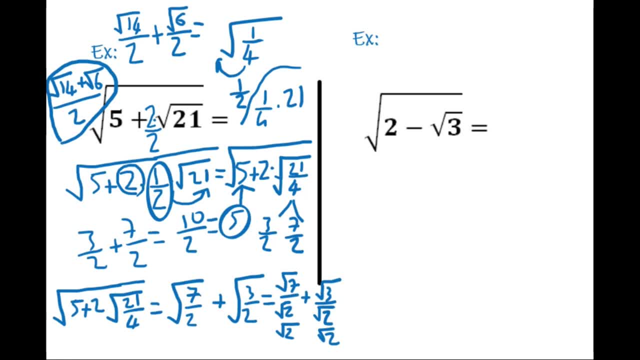 Now let's take a look at our last example. in this video, Again, We factor. before actually factoring these 3, there is a must, which is we have to put here 2.. Once you do it, you have to put here in the denominator part 4.. 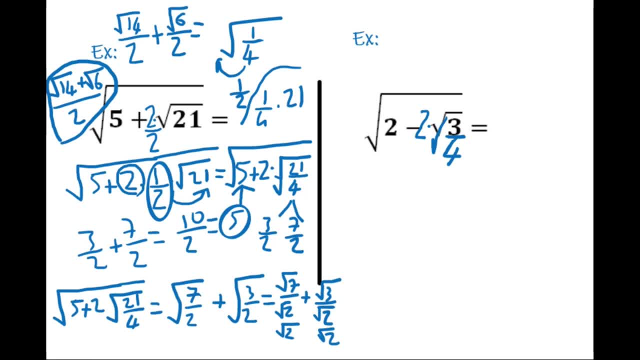 This is what we did in our previous example. So the question becomes 2 minus 2, square root of 3 over 4.. And now we can factor 3 over 4.. And we can write it as a multiplication of 3 numbers, 2 numbers. 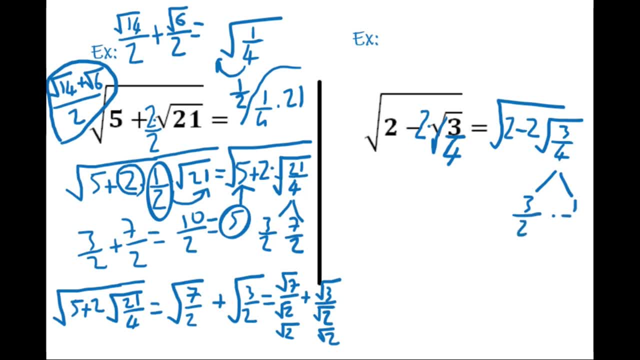 So 3 divided by 2 times 1 divided by 2 gives us 3 divided by 4.. So the result is: square root of 3 divided by 2 minus square root of 1 divided by 2.. Again, we have square root of 3 divided by square root of 2 minus square root of 1 is: 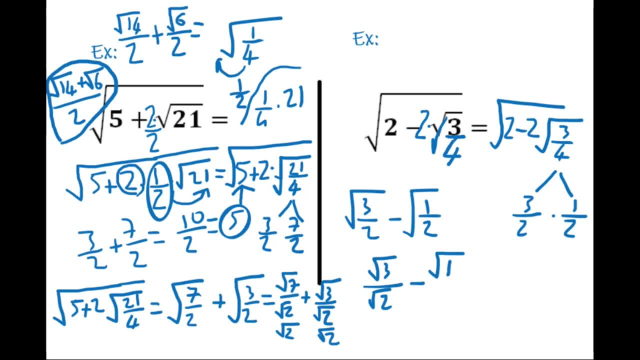 what- Let me write it first- actually Square root of 1 divided by square root of 2.. And again we need to get rid of the root from the denominators. In order to do that, we have to multiply numerators and denominators by square root of 2.. 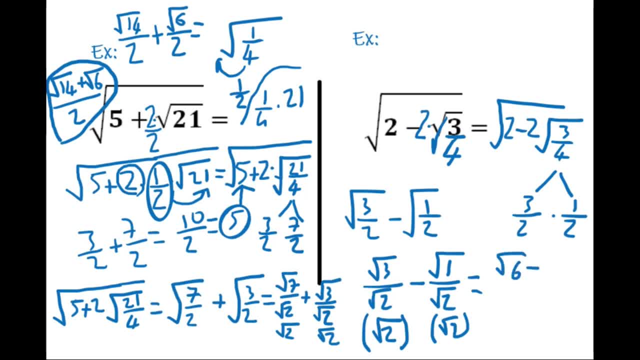 And once you do it you have square root of 6 minus this is already 1.. 1 times 2 is 2.. So square root of 2 divided by 2.. And this is the final answer. guys, Let's say you are in a test and there is such a question and you solved the question. 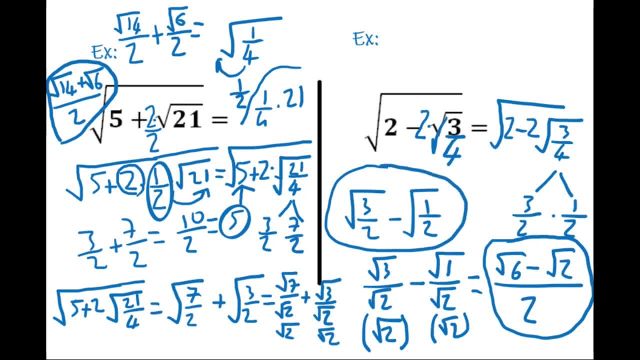 and you ended up this. But this one is not in the option. What you should do is you need to look for similar terms like, for example, this one and this one. They are equal to each other. Okay, But generally, this one, the final term. we can come across this final term, if there is. 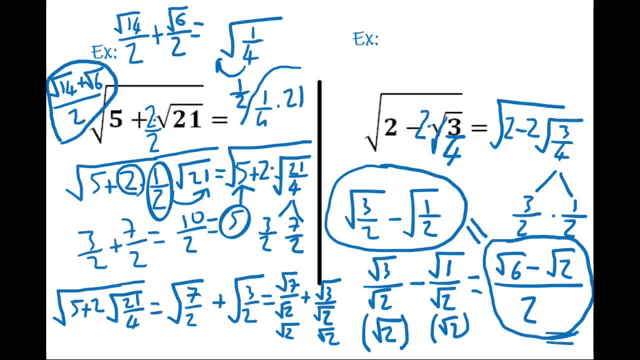 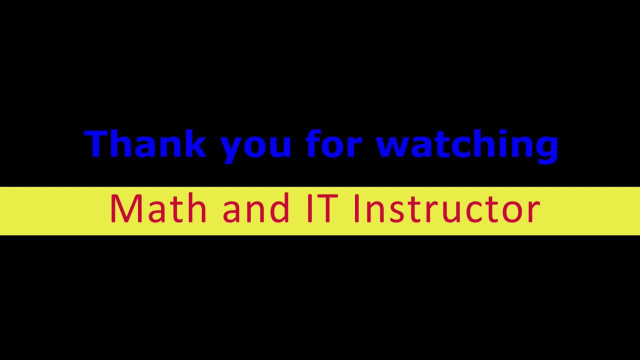 such a question. I'm planning to finish the roots and radicals topic. Okay, I hope you like it guys. Thank you for watching and hopefully see you in the next video. Bye-bye.